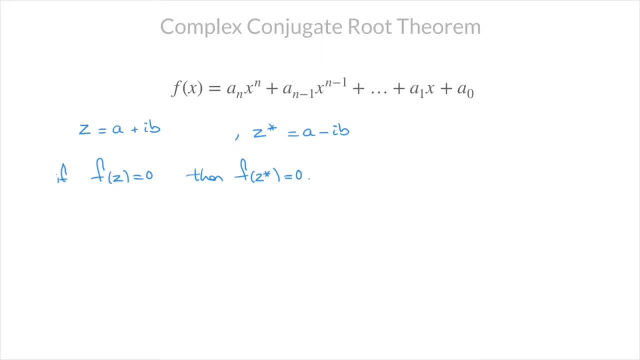 Now, what this actually means is that as soon as we have one complex root of a polynomial function, then we can state that its complex conjugate must also be a root. This means that complex roots of polynomial functions always come in pairs, For instance the polynomial function. 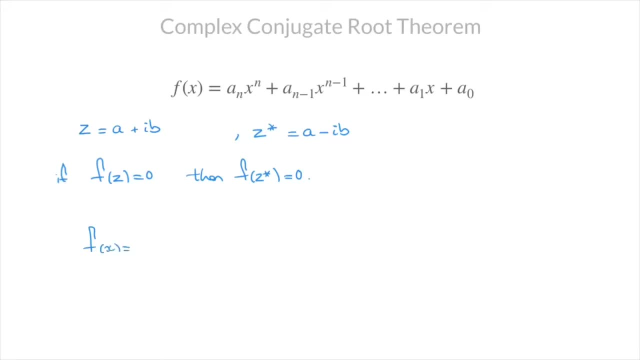 which I'll define as f of x equals to x cubed minus x squared, plus 3x plus 5.. One of its roots happens to be the complex number z, which equals to 1 minus 2i. Now, thanks to the theorem, we've just seen the complex conjugate. 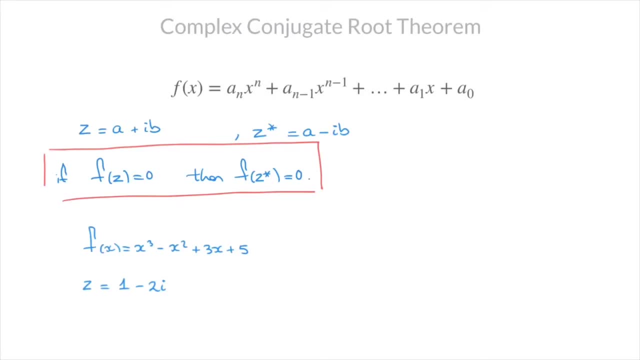 root theorem. we can go ahead and state without even thinking that because this complex number is a root of this polynomial function, its complex conjugate, which I'll call z star and equals to 1 plus 2i, must also be a root of this polynomial function. And you can go ahead. 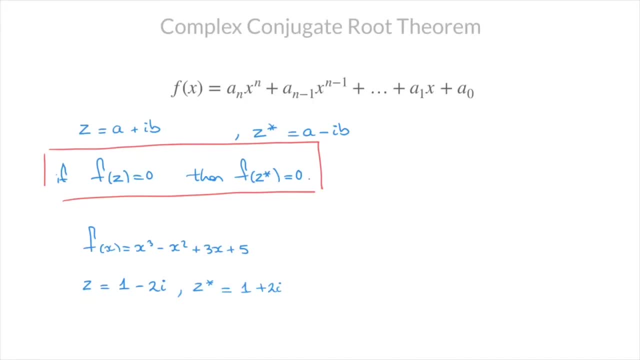 and check and plug in either z or z star into this polynomial function and you'll see that it will equal to zero. Okay, so that's the complex conjugate root theorem, And if that's all you were after, you can stop watching this video now, But if you carry on watching, we're going to work through a. 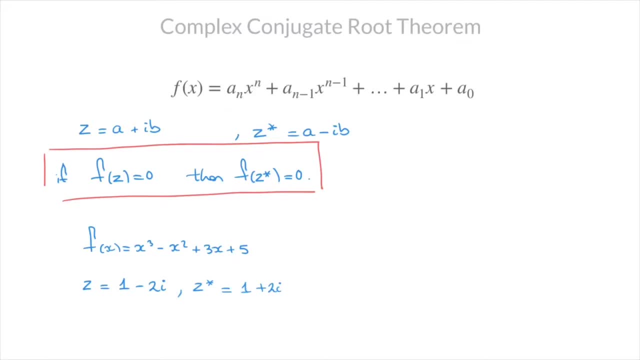 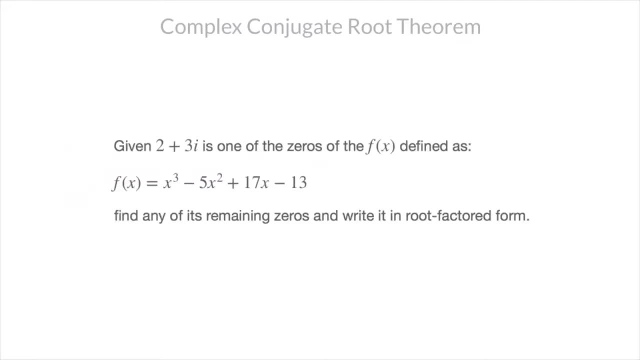 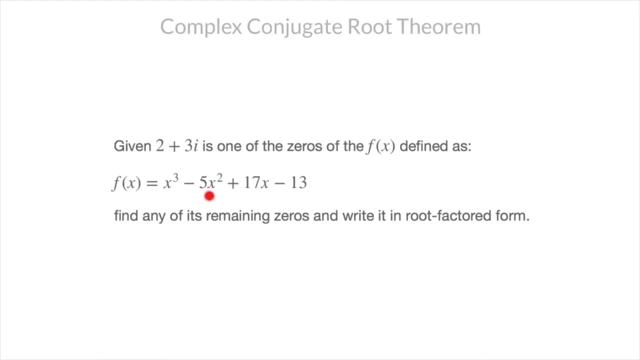 as f of X equals to x cubed minus 5x, squared plus 17x minus 13.. Find any of its remaining zeroes and write it in root factored form. Okay, well, let me start by moving this question to the side, Like so, And now we can get started. So, first of all, the question itself gives us: 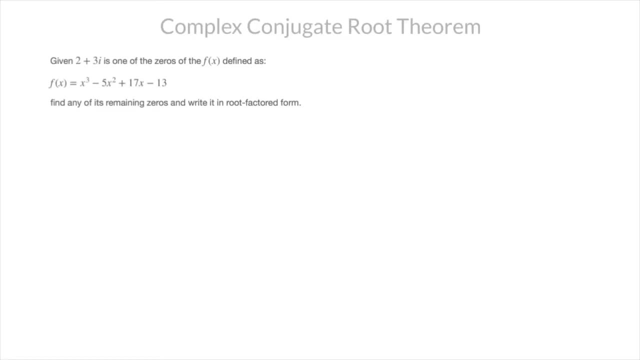 one of the roots of this polynomial function. Indeed, we're told that two plus three i is one of the zeros, in other words one of the roots. But now, since two plus three i is a complex number indeed, we could actually go ahead and write. 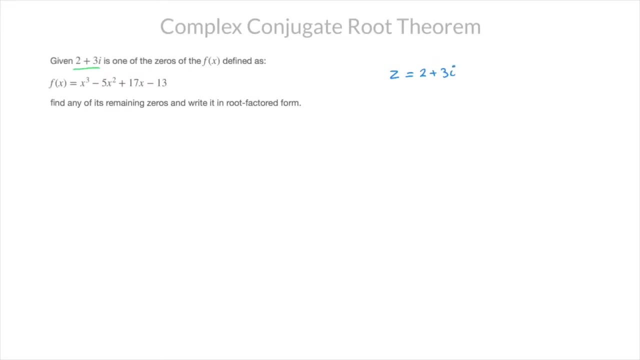 z equals to two plus three i. The complex conjugate root theorem tells us that its conjugate must also be one of the roots of this function, In other words, the complex number which I'll call z star, and equals to two minus three i. 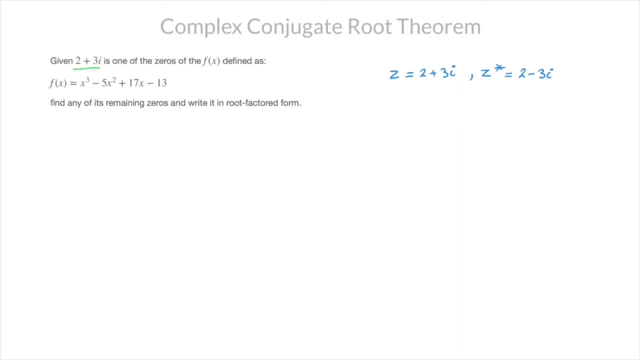 must also be one of the zeros of this polynomial function, And this means that we now have two of the roots of this cubic polynomial function. So how do we find the next one? Well, perhaps we could try finding it by trial and error. 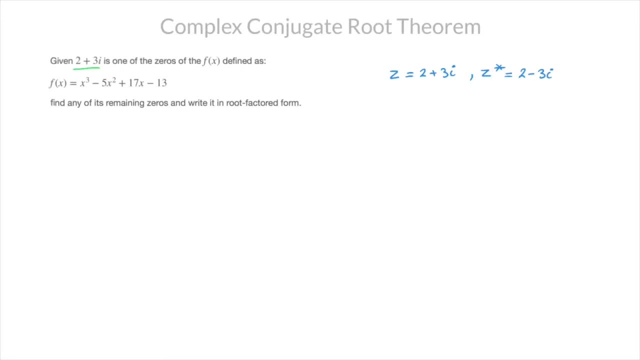 but at times that can be very tedious and definitely takes up time. No, instead we're gonna use the factor theorem. Now let me start by copying the polynomial function that we were given. Remember we have f of x, which equals to x cubed minus five x squared. 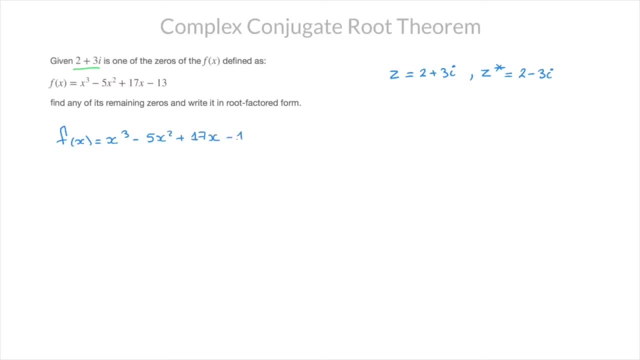 plus 17x minus 13.. And we've just seen that the two complex numbers, z, which equals to two plus three i, and its complex conjugate z, star, which equals to two minus three i, are both zeros of this polynomial function. 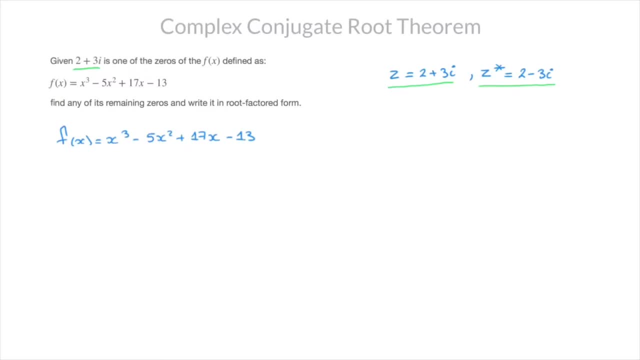 In other words, we can go ahead and state or remind ourselves that f of z equals to zero and f of z star equals to zero. But now, if we use the factor theorem for polynomial functions, the fact that z and z star are zeros. 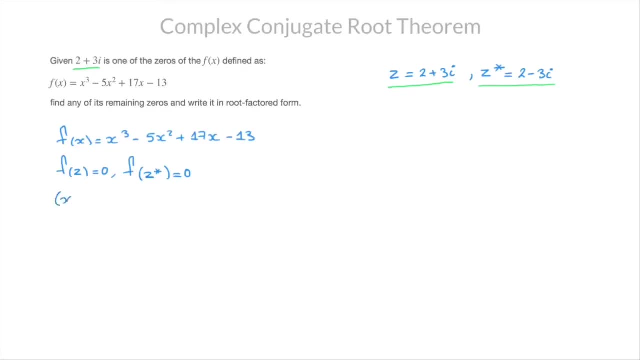 of this polynomial function tells us that x minus z and x minus z star are both factors of the polynomial function. In other words, we can rewrite our polynomial function- the one I'm boxing in gray right now- in the following way: We can go ahead and state that f of x 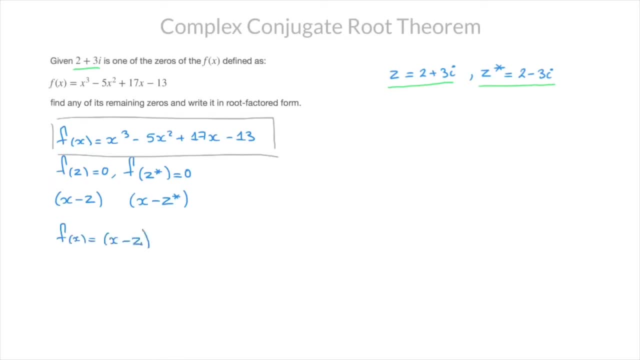 equals to x minus z times x minus z star times another function which we'll call q of x. And now the trick in finding the remaining root of f of x is to figure out what this function q of x actually is. And here's the trick. 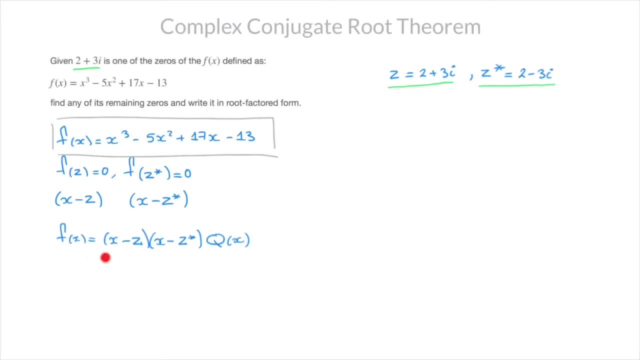 If we divide both sides of the formula, both sides of this equation, by x minus z times x minus z star, it gives us an expression for q of x. In other words, we can go ahead and say that f of x over x minus z. 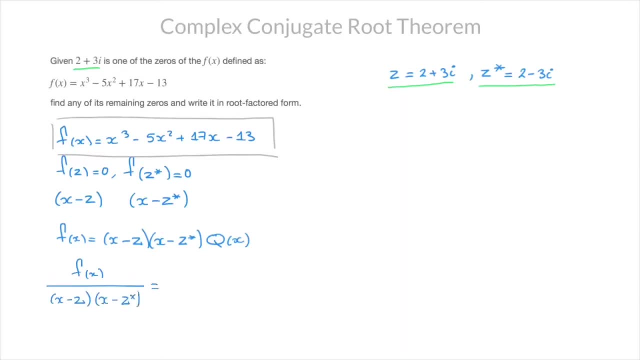 times x minus z star equals to q of x, So all we actually have to do to find q of x is to divide f of x by x minus z times x minus z star, Where z and z star are the two roots that we found at the beginning. 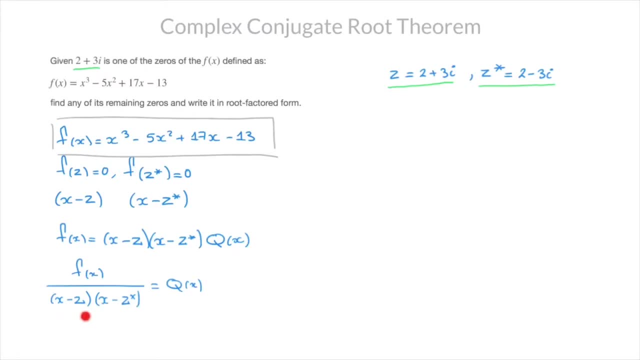 So let's go ahead and do that. The first thing I'll do is actually figure out what this product on the denominator is equal to. In other words, we have x minus z times, x minus z star. That's equal to x minus z, so z is two plus three i. 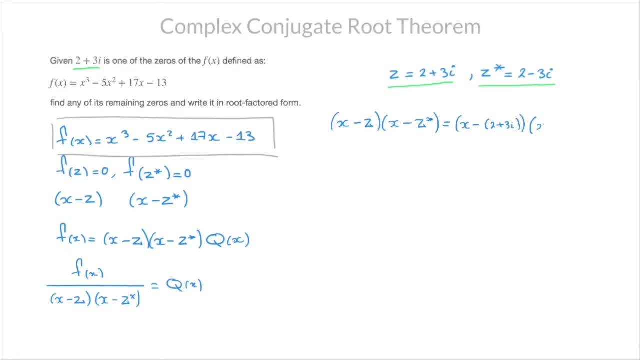 notice that I'm writing it in parentheses. times x minus z star, which is two plus three i minus three i Again, I write that complex number in parentheses. Now we distribute and in doing so we find that this equals to x squared. 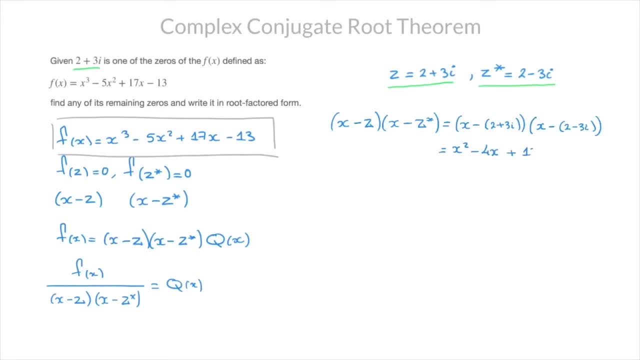 minus four, x plus 13.. And by all means, go ahead and press pause and check that for yourself. That should be the answer. So, going back to the expression for q of x, we need to divide f of x by this quadratic function. 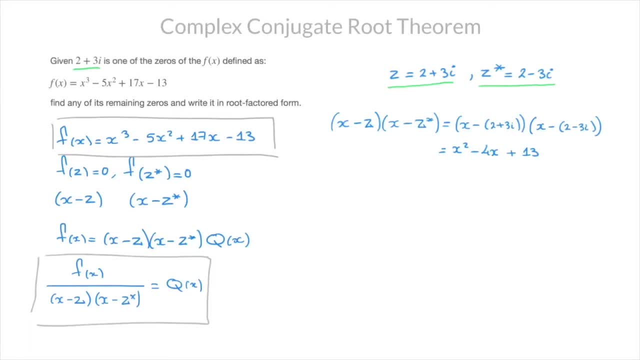 And to do that we use long division of polynomials. So let's go ahead. We're dividing f of x, which remember was x cubed minus five, x squared plus 17, x minus 13, by x minus z times x minus z star. 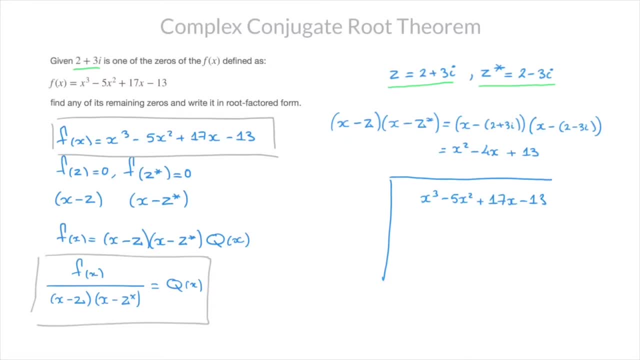 which led to the quadratic we found a minute ago. In other words, we're dividing f of x by x squared minus four, x plus 13.. Now to do this long division, we need to find what we'd have to multiply x squared by. 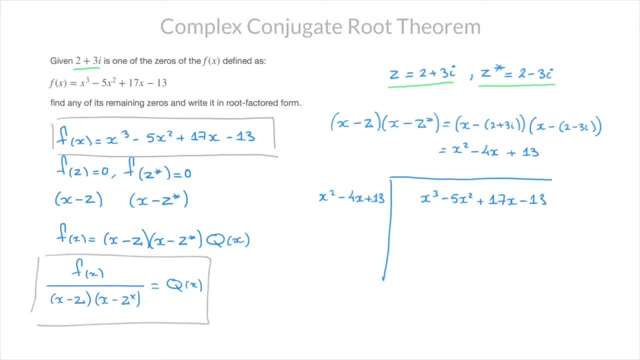 for it to equal to x cubed And it doesn't take us too long to see that that would be x. so I write x at the top And I now multiply this entire quadratic by x and write the result directly beneath f of x. 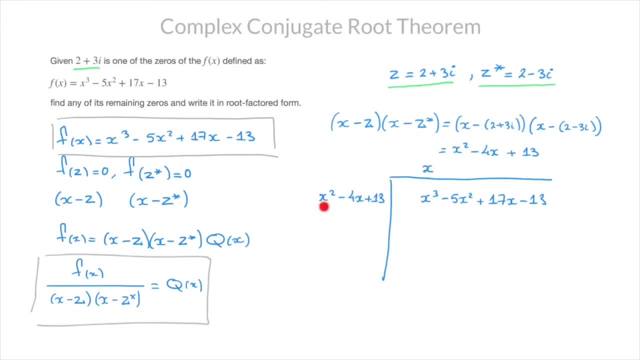 that we have here. So let's go ahead. We have x times x squared, which is x cubed. So I have x cubed here minus x times four x, which is four x squared, which I write directly beneath the five x squared there. 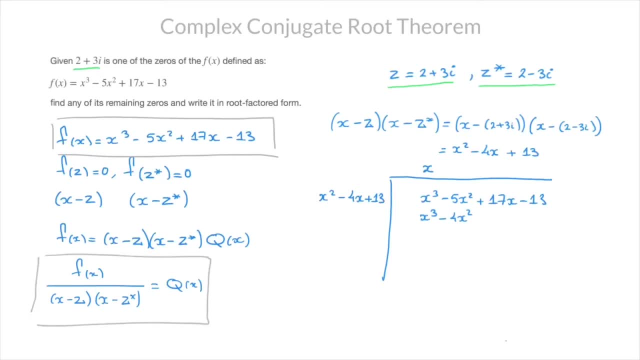 plus x times 13,, so that's 13 x, which I write right here, And I now subtract this entire result from f of x, like so. So I have x cubed minus x cubed. so that's zero negative five x squared minus negative four x squared. 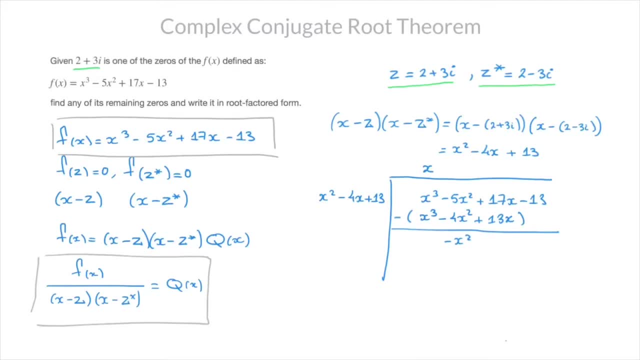 so that's negative x squared and 17 x minus 13 x, which leads to four x, And finally I carry down this negative 13.. So I have negative 13 at the bottom here. Now that that's done, I repeat the process. 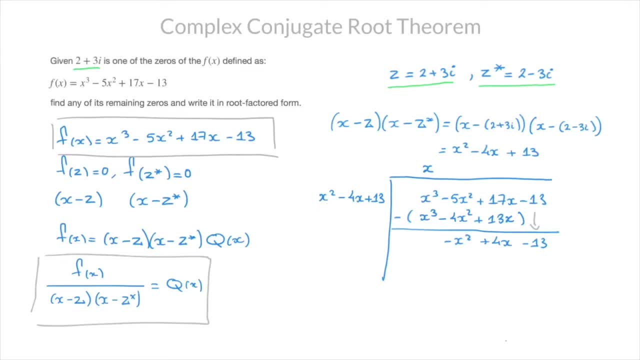 and figure out what I would have to multiply x squared by to get to negative x squared. And it doesn't take us too long to see that we'd have to multiply x squared by negative one for it to equal to negative x squared. So we write minus one at the top here. 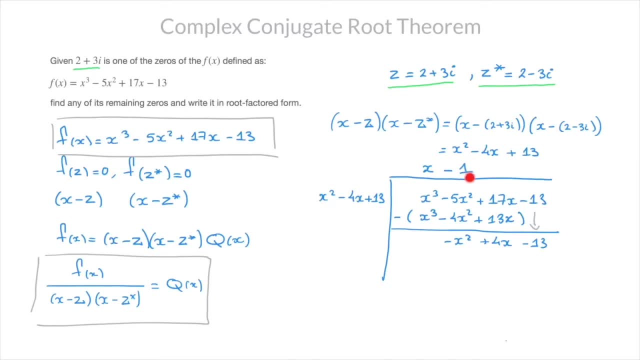 We now multiply this entire quadratic by negative one and write the result directly beneath the quadratic that we have here. So let's see we have negative one times x squared. that's negative x squared, minus negative one times four x. so that's minus negative four x. 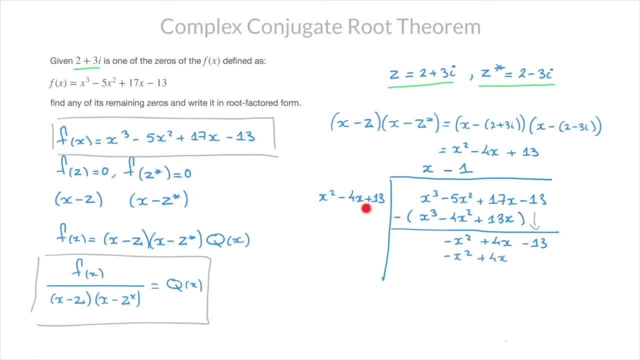 in other words, that's plus four x, plus negative one times 13,, so that's minus 13.. And now, subtracting this result from the row above it, we quickly see that this equals to zero. And this zero tells us that, when we divide f of x, 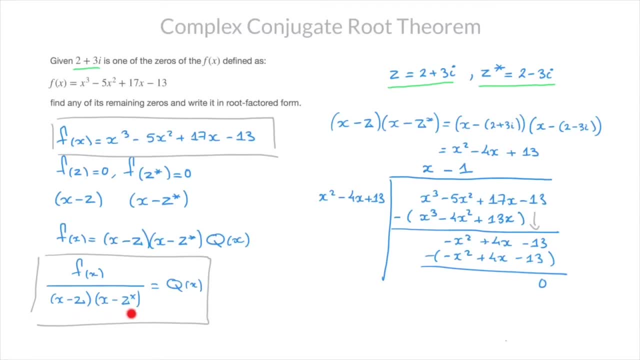 by x minus z times x minus z star, the remainder is zero, which confirms that these are both factors of f of x. Most importantly, though, at the top of this long division, we have our function, That's q of x, the quotient function. 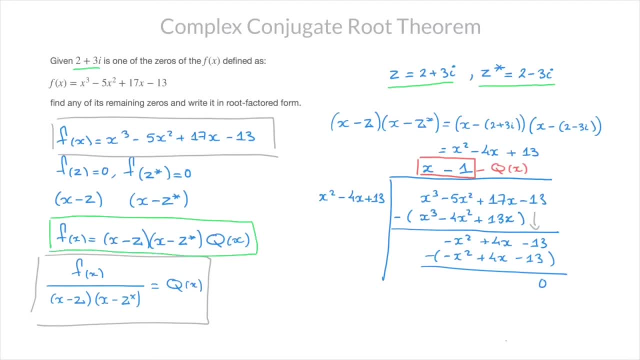 And going back to the result that I'm currently boxing in green, we can now state that f of x is equal to x minus z times x minus z star times x minus one, Or going further and replacing z and z star by their respective values.